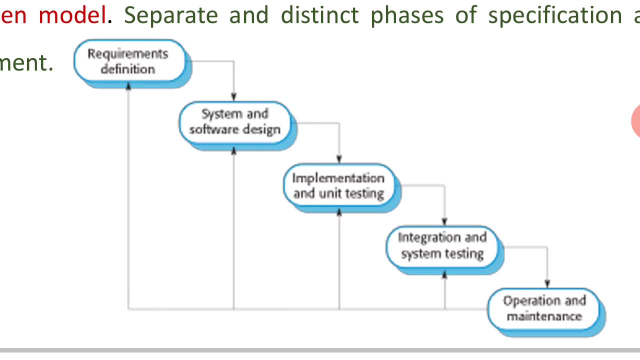 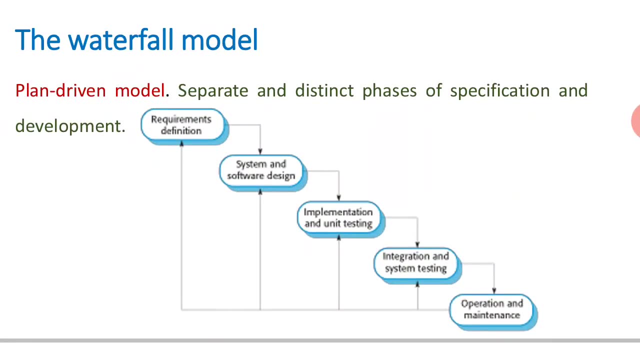 The third phase. So, like this, the process will be taken over here, okay? And another important thing is, just do remember, in every software process model, including this waterfall model is concerned, okay, always do remember our we will be carrying out the same four fundamental process activities. 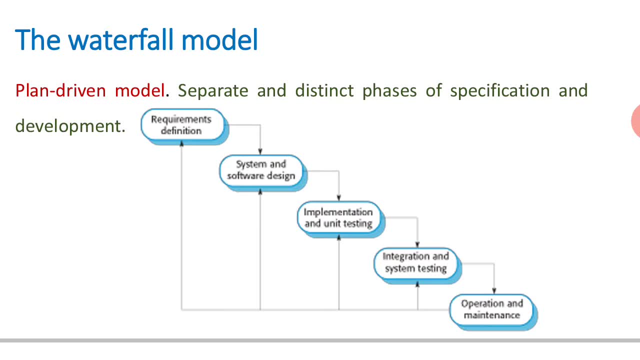 always remember. what are those? software specification, design and implementation, software validation, then what? software evolution? the only thing is, the way of carrying out these activities may be different. based on that, my software process model will get changed. so here also, in the waterfall model, we are going to carry out the same activities. 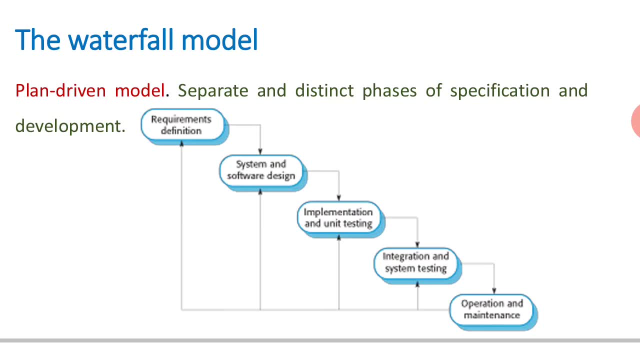 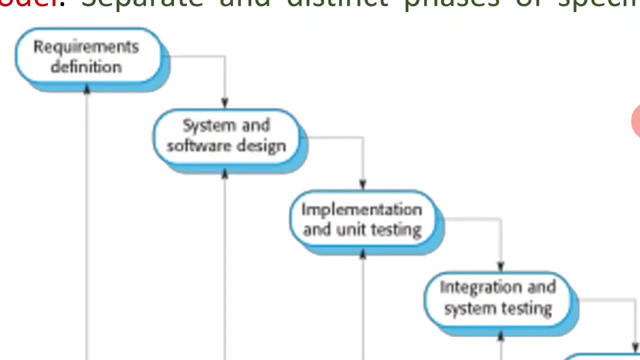 but in a in one particular approach is clear. so just have a look at here what are the different phases that we have identified for waterfall model. so my first activity, or first phase, is: what the requirement definition. then second one is a system and software design. third one is: 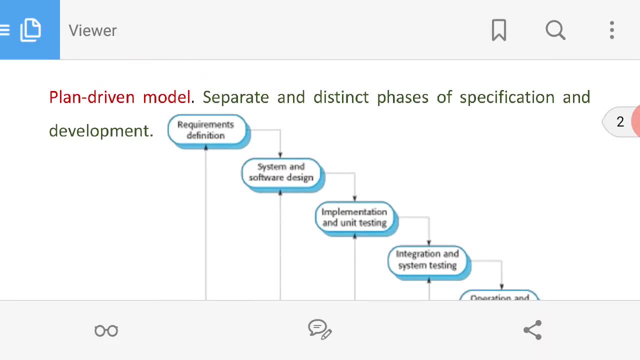 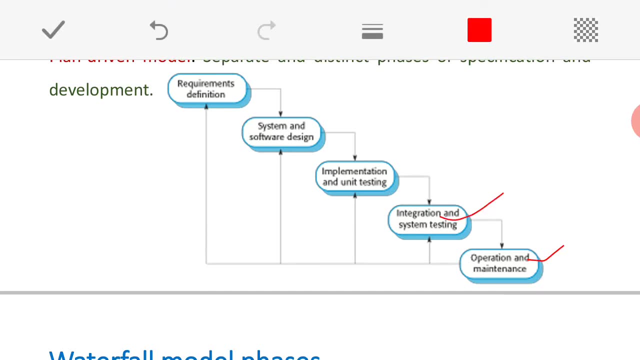 implementation and unit testing. okay then, fourth one is what that is? integration and system testing. and last one is operation and maintenance. so these are the, say five different phases that we have identified for the software, this waterfall model, but when you combine all these five, they are nothing but a part. 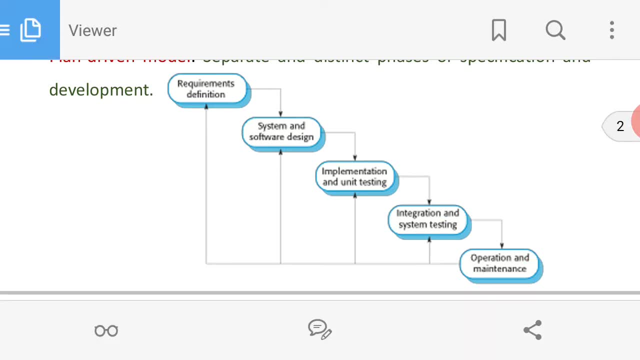 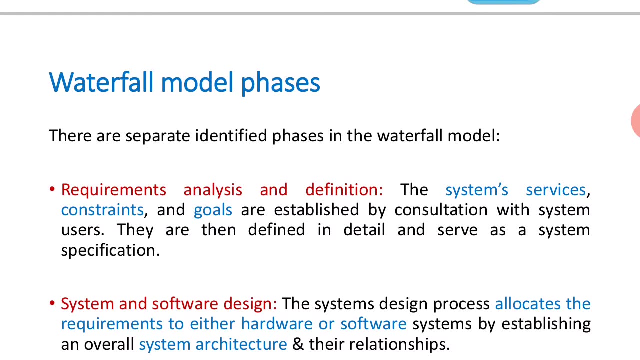 of our four fundamental activities. okay, so just we will see one by one all these phases in detail, what exactly we are going to perform in all these different phases of this waterfall model. so the very first one is: what requirements, analysis and definition. so in this particular phase- just have a look at here- so we are going to establish. 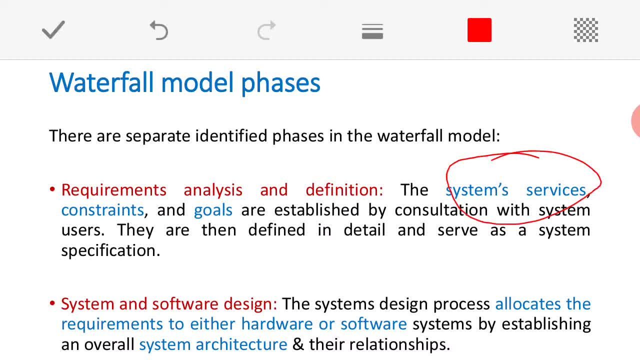 the system services. what are system services? system services are nothing but what the functionalities that my software is supposed to what provide to the end users. they are nothing but what system services or the requirements- okay, what my system is supposed to do for my customer. okay then constraints. constraints are nothing but what? some sort of rules and regulations based on. 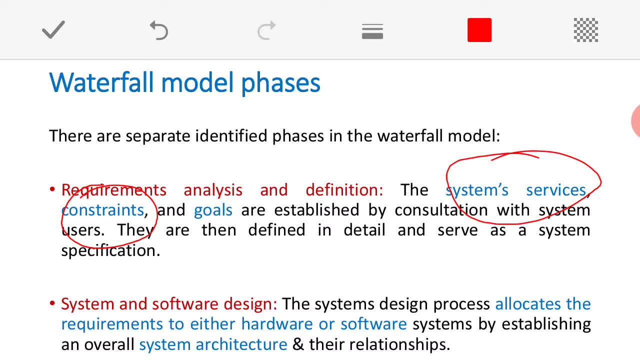 which i am supposed to develop the software. okay. so either it may be a technical related constraints or it may be non-technical. see, for example, say, budget constraint- how much money that i need to time constraint- okay, with what? within within what deadline i have to develop this software as a 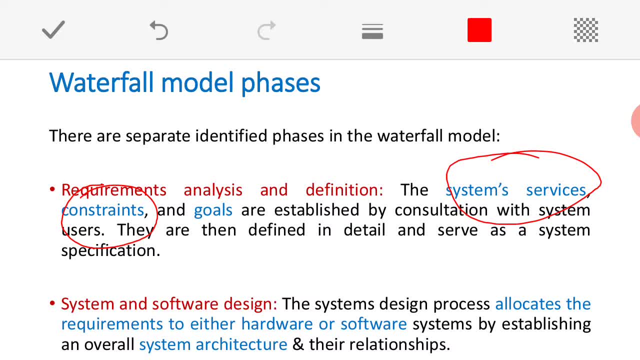 project. okay, so it may be human resource constraint. how many investment constraints? so what are the constraints of this software? so, in talking about this software- owned sensors against the الع correlating to the underlying system- we have a law according to which employees that i need if i start developing this particular software. is it clear then? what about? 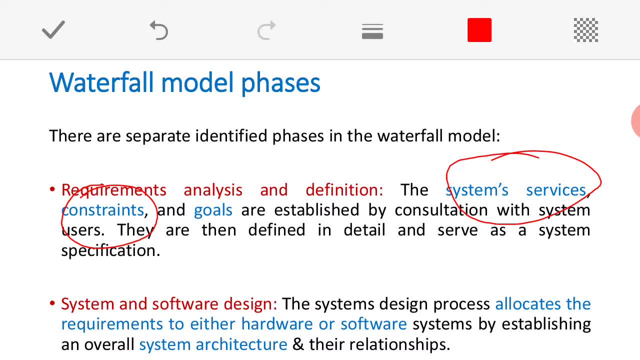 the technical constraints means non-functional requirements. what about the quality of the software, speed, execution, okay, so all these things will come into picture that we need to what establish and also we need to establish what the goals with respect to management perspective, with respect to the organization perspective, okay, whether it is a profitable or not, how much? 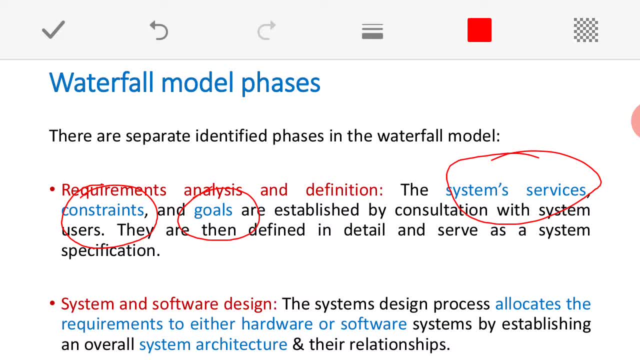 profit, we will get it. what brand name you can get it? okay, all such things that we need to establish. okay, how it will be get established by consultation with system users, who are the system users here, the end users or the customers or any stakeholder who are directly or indirectly related to that. 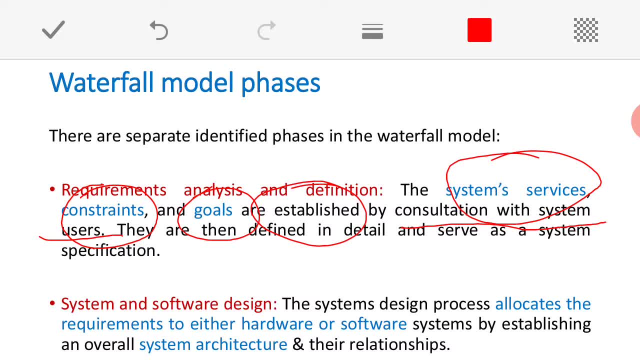 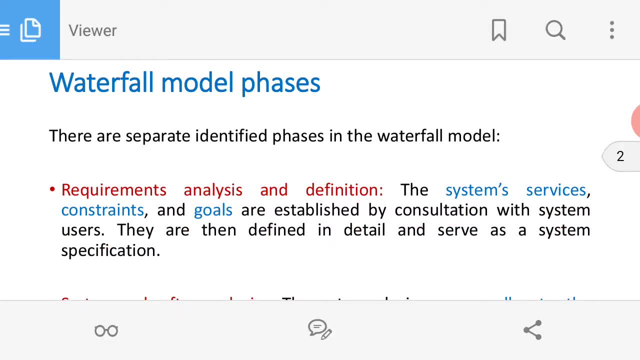 particular software system that we are planning to develop. it is clear, okay, so all these things should be get defined and those requirements should be defined, and so these things should be defined, and so all these things should be be finally converted in terms of what, the detailed specifications, so that we will discuss. 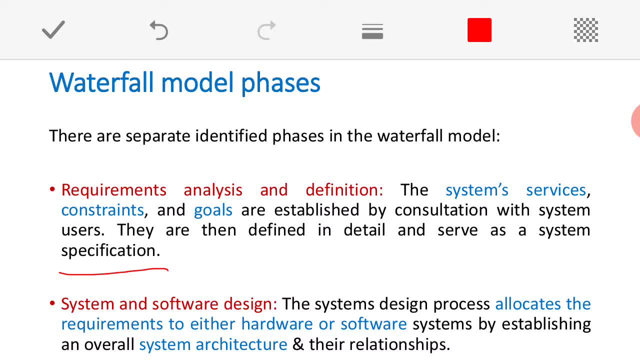 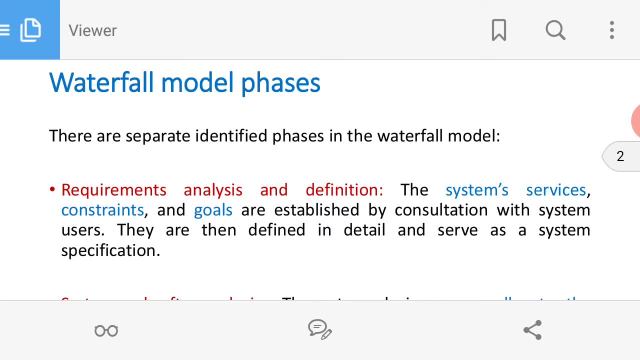 it later how we are supposed to define the requirements in terms of what software specification there are. different methods and concepts are available. that we will learn it in the forthcoming chapters. clear, so once this is the first phase, ok, so once I will finish this first phase, I will move on to the second phase. what is that? so, once my requirements are defined, I 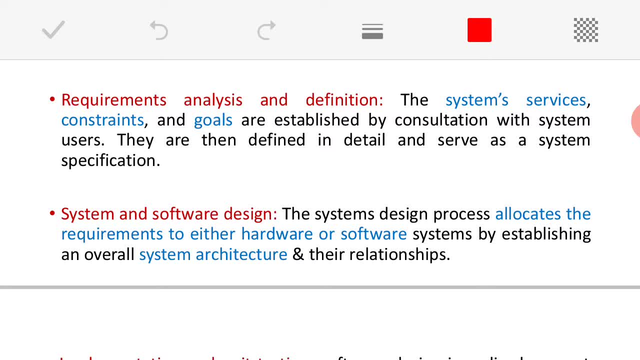 will go for second one, that is, system and what software design? see there, I am using two words here. ok, I am not talking about only software, I am also talking about what a system. when I am talking about a system, it is not purely software. it is combined both hardware. 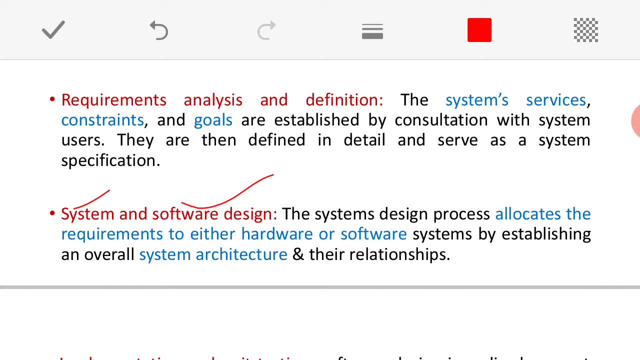 plus what software? because to run any software I need a support of what hardware. that is the reason that normally we used to consider software- also what- as a system. ok, so system and software design. So in this design, This part is concerned here. look at there. in this particular process we are going to 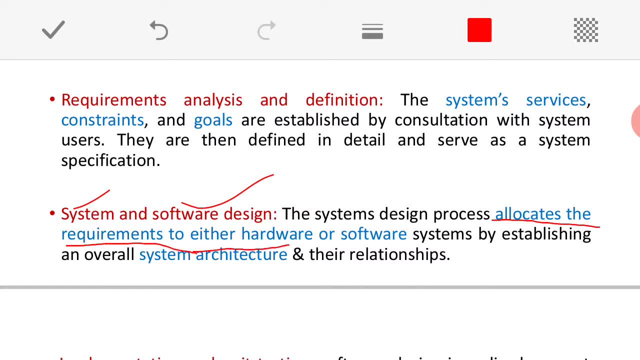 allocate the requirements to what? either hardware or what software system. why? because my system consists of two parts: either hardware related or what software related. here I have defined my requirements. now what I will do: I will bifurcate which requirements are related to hardware and which requirements are related to what software, so that I will make an allocation. 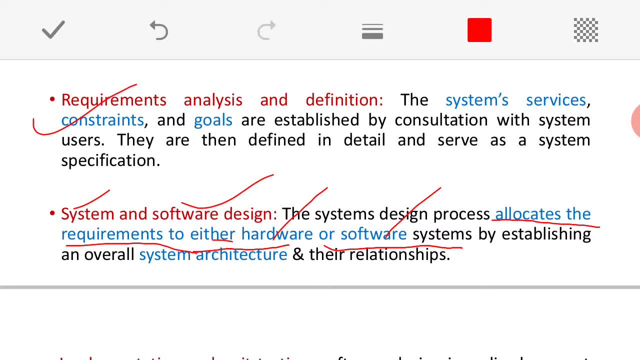 ok, and after doing that, I will establish The overall system architecture. that is nothing but what, just in the design. just try to recall overall organization of what my system? why? because we have already told system is not a single entity. it is made up of what? different components or different subsystems? then how? 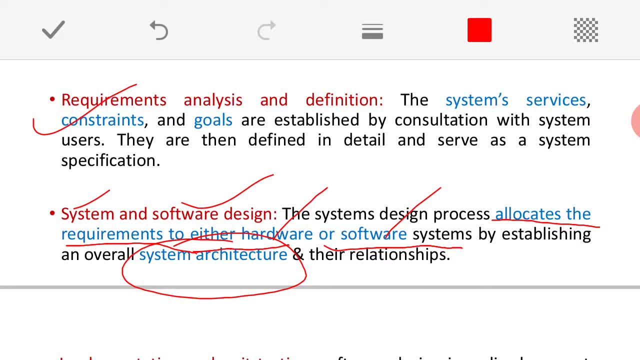 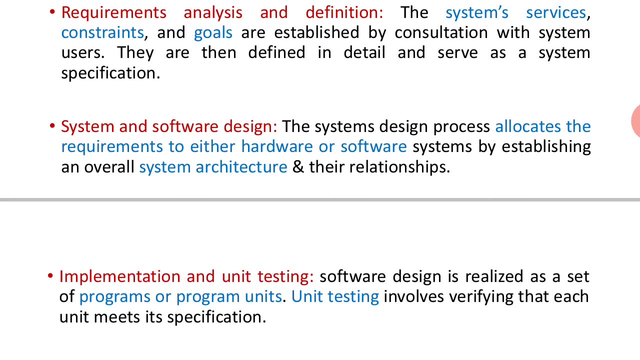 I am going to make arrangement how all these parts will be get interfaced. for that I am going to define what a system architecture and how those parts will be get what interfaced with what relationship, ok, Ok, that we are going to what define. ok, so this is my second phase, so after completion. 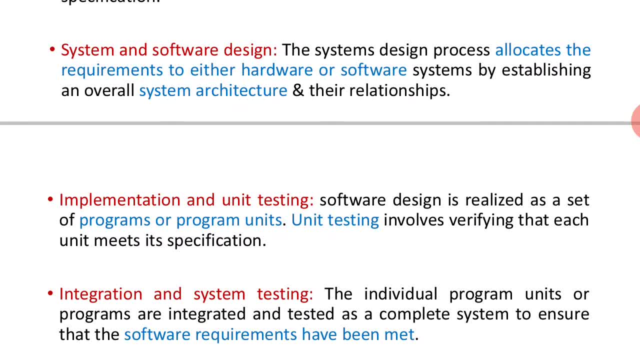 of the second phase. I will start with what my third phase. what is the third phase? that is implementation and unit testing. so once my design is ready, architecture is ready, I will work that design in terms of what? the program, so writing program, is nothing but implementation. see there, my software design is realized as a set of what programs or program. 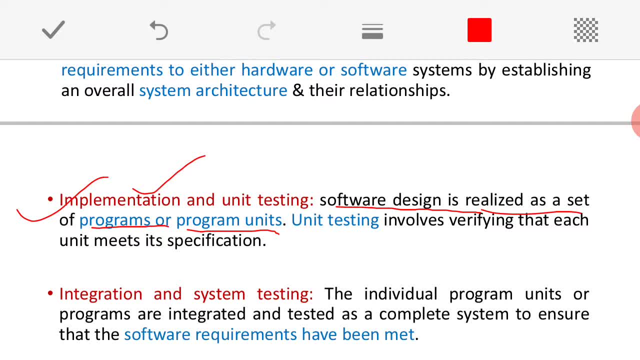 units. So here every program is known as what one unit? is it clear? ok, so like that, I will write n number of programs as a units. when I will combine all those, n number of programs, I can call it as what? my software system. is it clear? so that is called implementation while doing. 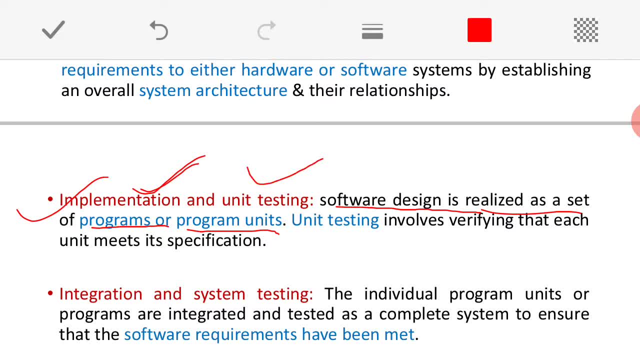 that implementation itself. look at there, we are going to carry out another activity here: unit testing. what is unit testing here? every unit is known as what a program. that you remember, ok? So, anyway, we are going to write n number of different programs, and every program is: 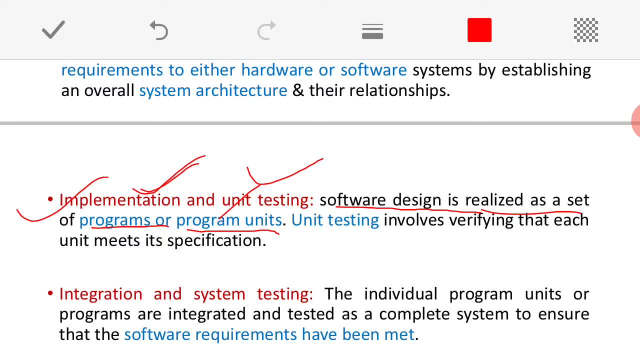 written by one developer or any software engineer and this is the responsibility of that software engineer to validate or test his program. if I am writing one program on salting, it is my responsibility to check what input I am supposed to give and what is the expected output why? because I have written the program, I know the logic, so like that, 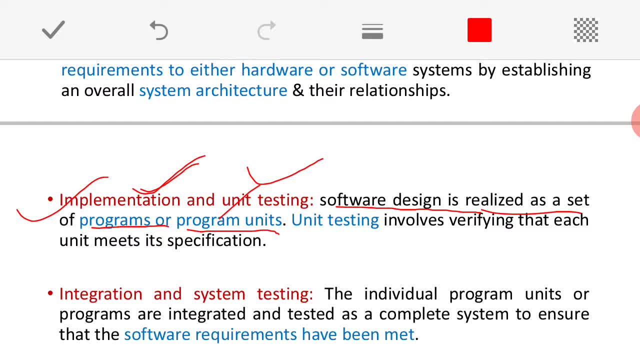 if there are fifty programs, fifty people will write the program and they they will perform a testing on those fifty programs. that is called as? what? a unit testing, is it clear? so, program by program, I am going to perform what the testing here. that is called unit testing, and it will be done at the time of what implementation itself. is it clear? so, 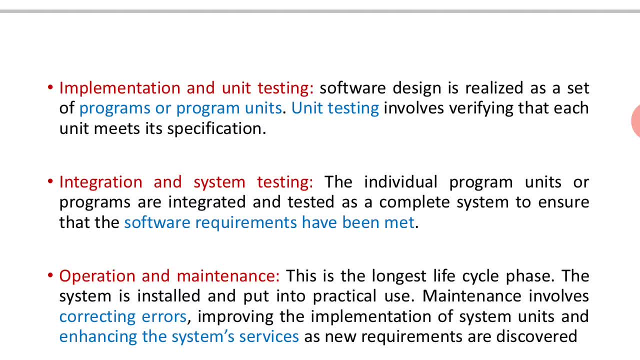 after doing that now we will go forward, the next phase. the next phase is called as what? integration and system testing. ok, just have a look at here. in my previous phase. always do remember, in every phase there there will be some output. Ok, So in my previous phase here, ok, what is the output of my previous phase? so I have written. 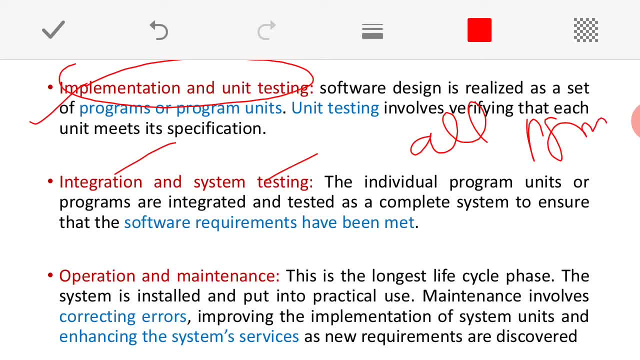 all the programs, ok, and all these programs have been what tested? is it clear? now I will go forward. integration: all these individual programs will be individual programs, nothing but what units that will be get what integrated. when I will integrate all these individual programs, what I will get? a complete system. and once again I have to perform what testing? 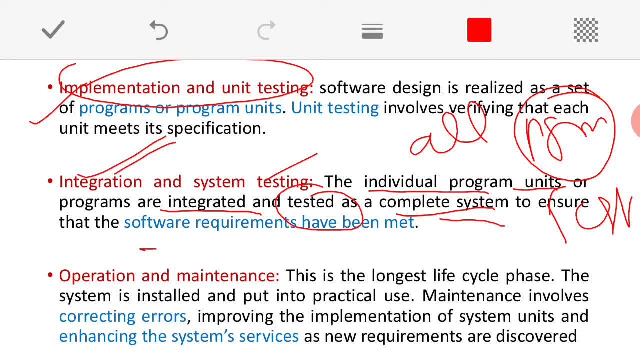 I will get a complete system. ok, for what purpose? to check for whether the system requirements have been met or not. what are system requirements? system requirements are nothing but what specification that I have defined in what my first phase? ok, try to recall here. see there, so this is. 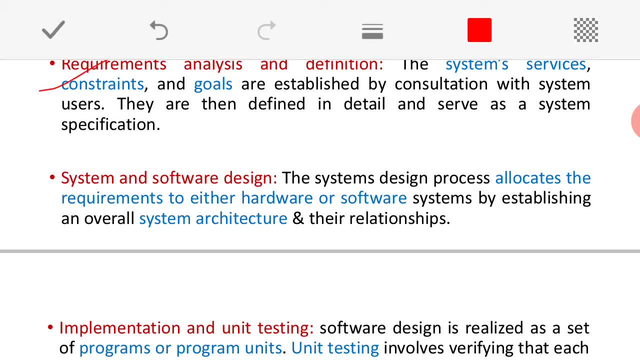 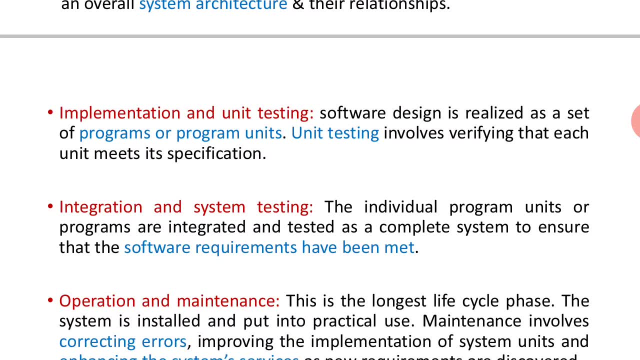 my first phase. so here I have defined all my specifications. ok, so once my software is ready I have to test of in a system testing. I should conclude that whether my all requirements have been met. What are requirements? requirements are nothing but what the customer needs: customer services. 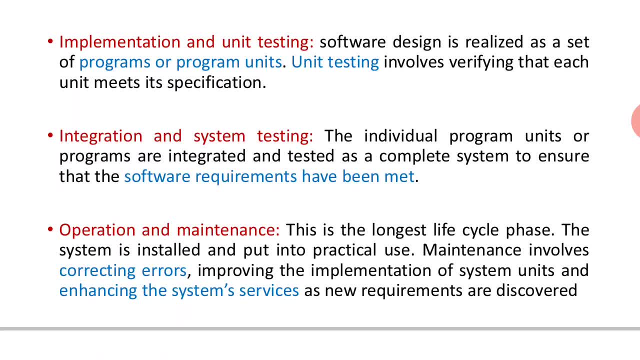 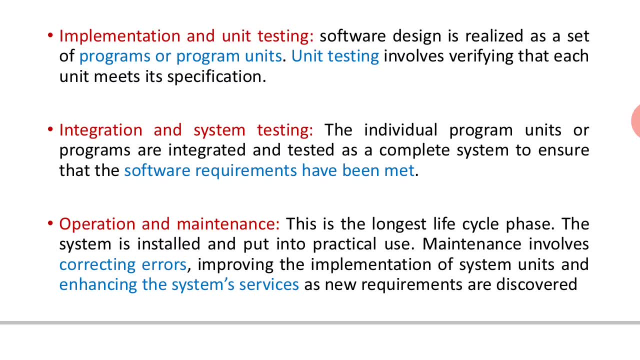 what the customer is expecting. that we need to confirm. ok, so once my software is ready, I have integrated. once again, I have done the system testing on the whole. is it clear? ok, and another important thing is- you may get the doubt here, anyway, we have done the testing. 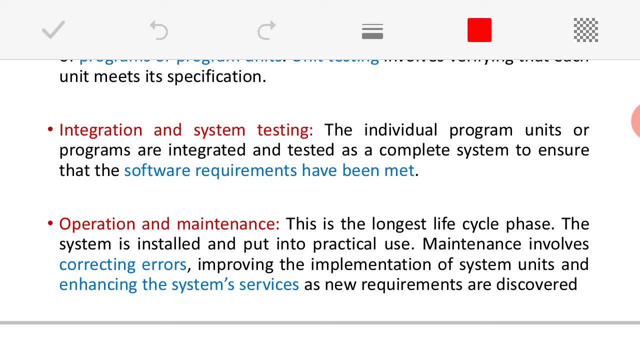 on individual program, why we need to do once again after combining the program, why we need to do the testing here. always do remember it is very simple: See, when you have tested P1, it might be ok. when you have tested P2, it might be ok. but 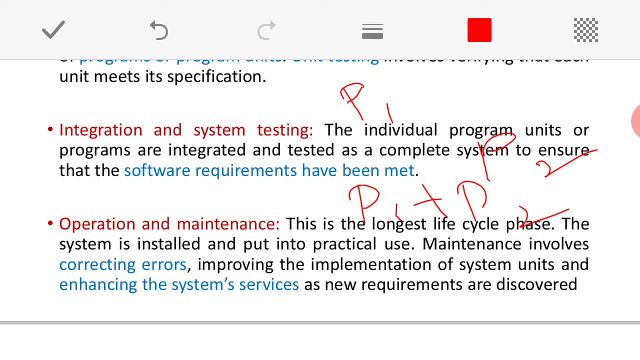 when you will integrate P1 plus P2. it is not compulsory that you should get always the correct output after integration. there may be some errors or some bugs. so that is the reason that, even though if you have tested program by program, unit by unit after integration, 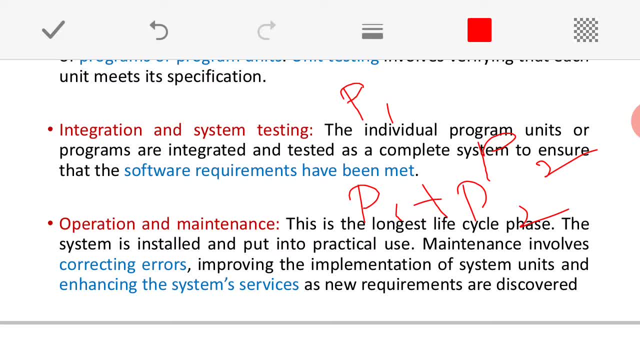 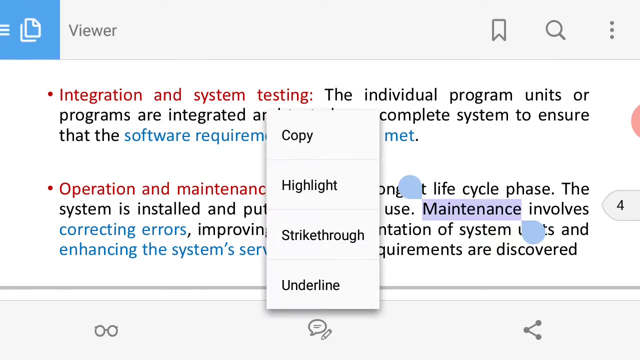 once again, after completion of your whole system. you have to perform the testing on the whole system. if your whole system is working fine, with proper as per the specifications, then you can say that, yes, your software is what ready and it is get tested. ok, so once the software is ready, now we will go for the last step. just have a look at there, what is? 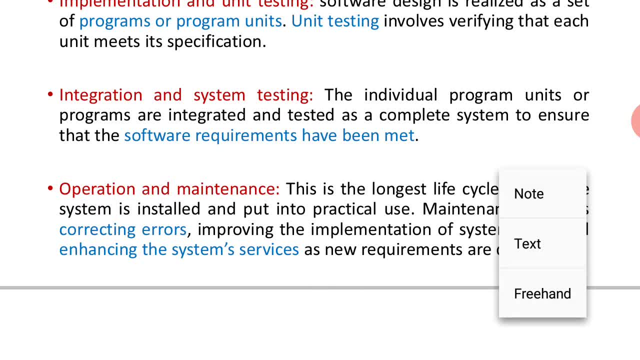 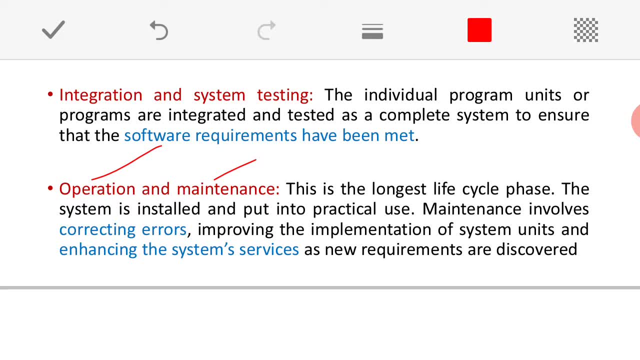 that last step here, that is, operation and maintenance. ok, so once my software is ready with validation is completed, That will be hand over to the customers. the customer will start using that how, the how it will be get delivered to the customer. the system is going to what installed and it will. 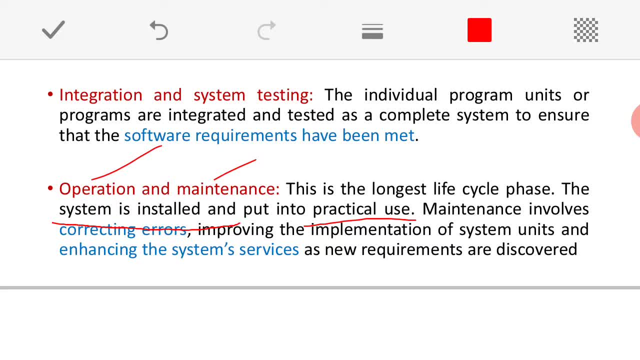 be given for what? the practical use? practical use in the sense what the customer will start using that software. is it clear that is called operation once the customer will start using that software automatically. they might be, they may get some bugs, some errors in later stages. is it clear? 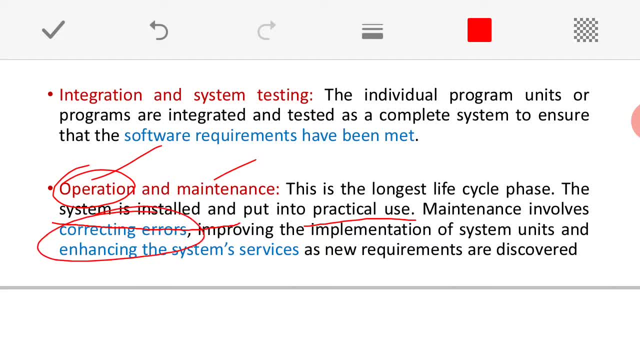 They may get some errors, Ok. Or after started using the system after few days they want to enhance the system service. enhance the enhancement of system service is nothing but what the modifications? they want to add some new requirement or they want to make modification for the existing requirement. 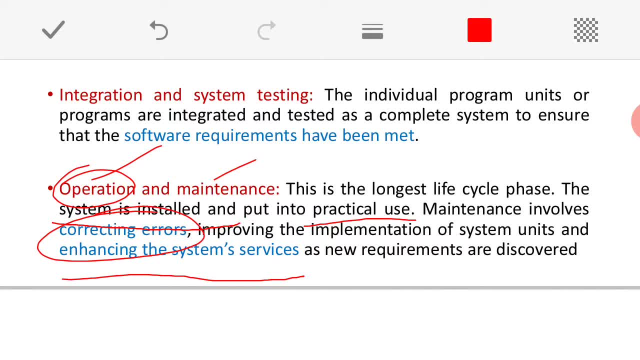 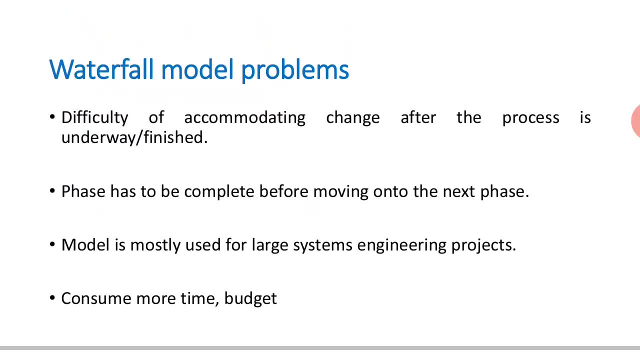 or they want to delete some unwanted requirements. that is nothing. but what the maintenance or what the evolution is it clear? So this is what taking place in the last step. ok, hope all of you understood all these five steps over here. then finally have a look at the advantages and disadvantages of this. 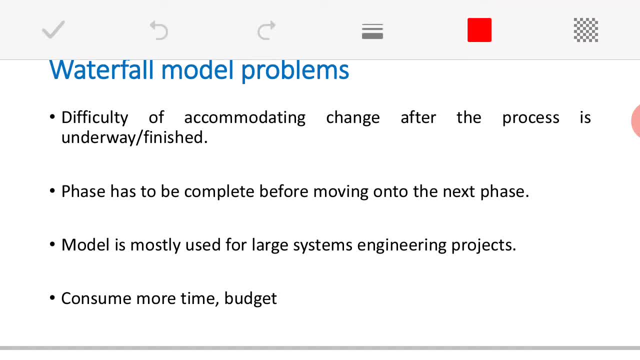 waterfall model is concerned. ok, the very first problem or disadvantage that we can mention over here is it is very difficult to make the changes or accommodate what the changes into the process of this waterfall model once it is get started or it is get what finished. why? because, do remember, waterfall model is a very strict model. it is a very 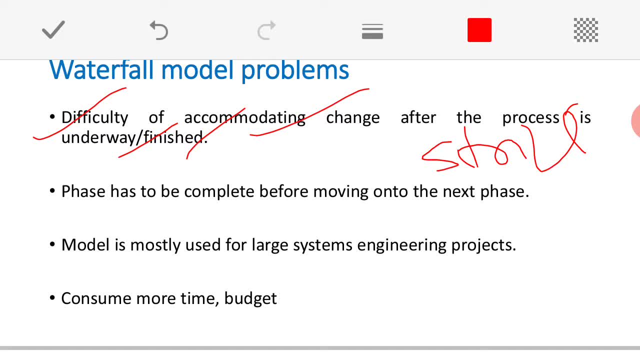 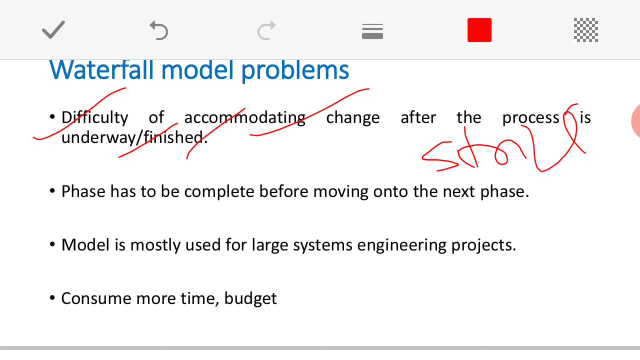 the second phase. once you will complete the second phase, then only you can go forward the third phase ok, while moving towards, like that, after reaching the fourth phase. if you come if any changes to be taken place in the first phase, then it will be very difficult to do. 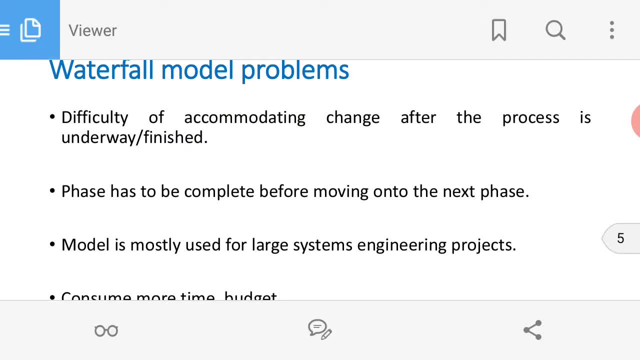 that is it clear? ok, and the another point is: see there, that is the reason that we say that phase has to be complete before moving on to the next phase. That is the reason that we told that it is a very strict phase. it is not. it is not flexible. 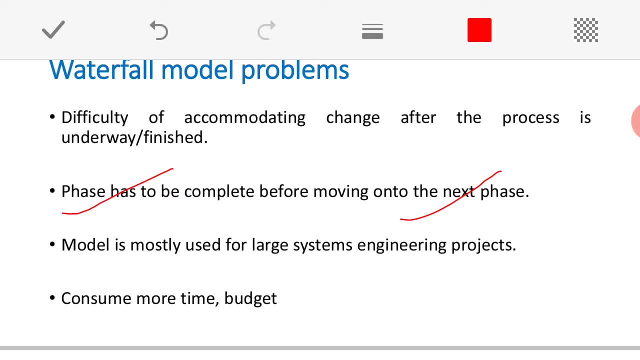 at all. it is not a flexible at all. ok then, this model is mostly used for what large engineering projects? it is suitable only for what large scale software systems? ok then, last one is: it is going to consume more time, more budget. ok, even the effort, man power, everything is. 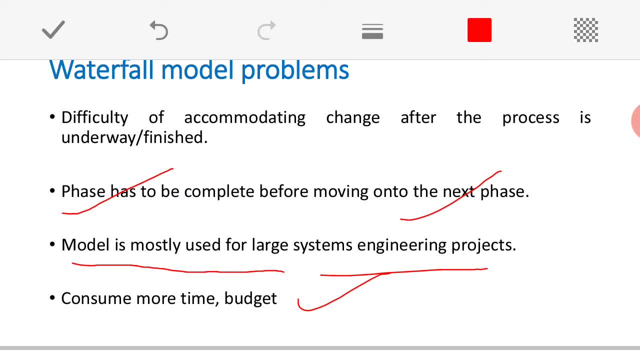 more here because, as it is a strict model and also which is applicable mainly to the large scale projects, automatically to complete those projects it requires lot of time, lot of money, investment and all those things. ok, and the very important thing is see there: whenever you want to go with this waterfall model for your software development, make sure. 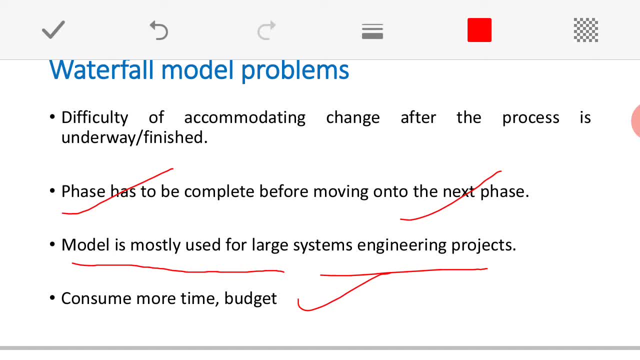 that you are 100% perfect in your requirement definition, in the very beginning itself. if your requirements are well defined and if they are 100% perfect, then only you can go forward this one. Otherwise, every time after going after completion of design and implementation, you cannot come.